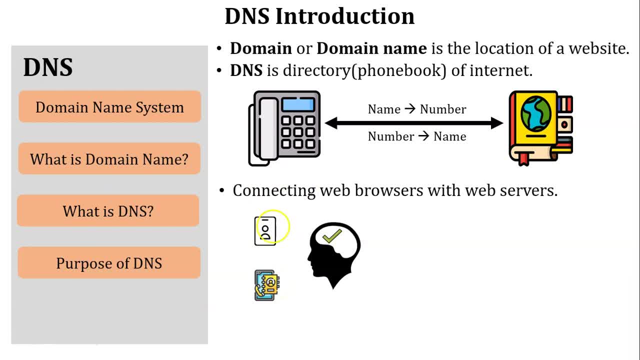 we can remember the as many as person name. So as we know that we are stored the number with particular person name. So, on the same way, someone ask you to open the Google and Facebook using the IP address, So our brain can remember the limited number of IP address. 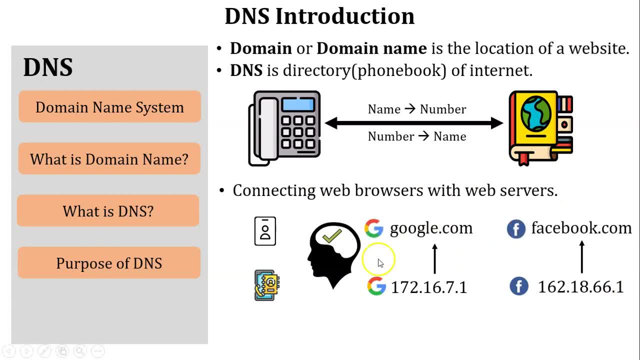 So we are accessing all the website using the website name instead of IP address, Because human brain can remember the maximum website names instead of IP address. So the purpose of DNS is mapping IP address to the naming and naming to the IP address, So it is the same as telephone directory. 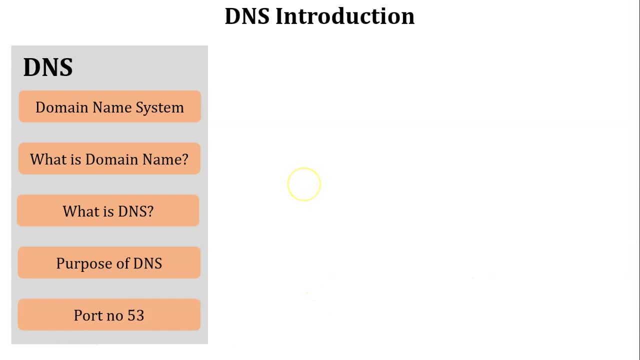 Next, DNS uses port number 53. So the process of DNS using the port number 53, with UDP protocol and with TCP protocol. But in the working of DNS UDP protocol is the default protocol Because in DNS immediate response is required to the user. 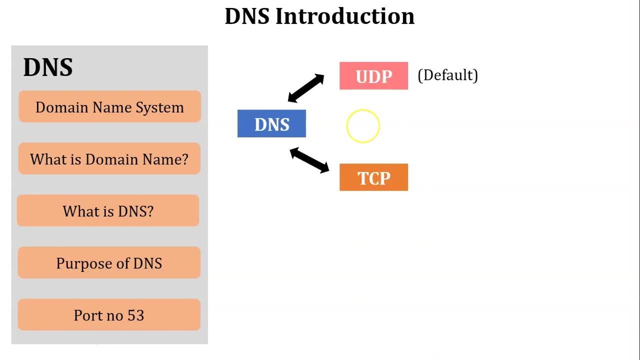 So UDP is faster in compared to TCP, So UDP is the default protocol of DNS. So here there are two question in my mind. The first question is: why does DNS use UDP instead of TCP? The another question is: in which case DNS uses the TCP instead of UDP? 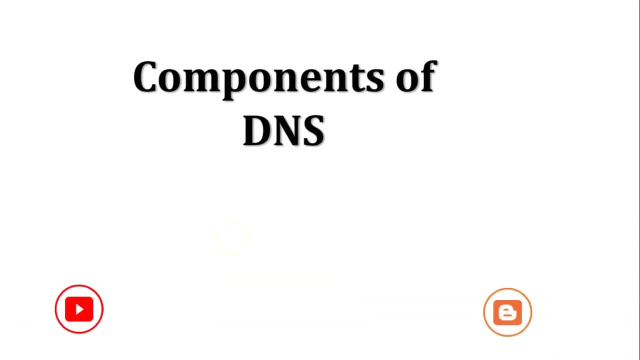 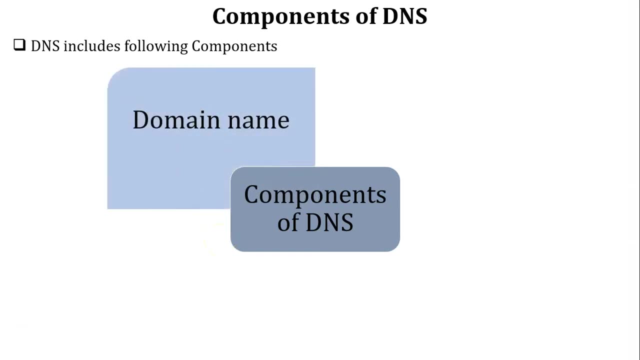 So write your answers in the comment section. Next, components of DNS. DNS includes the following components: The first component is domain name, The second one is namespace, The third one is name server and the fourth one is name resolver. Now discuss all the components. 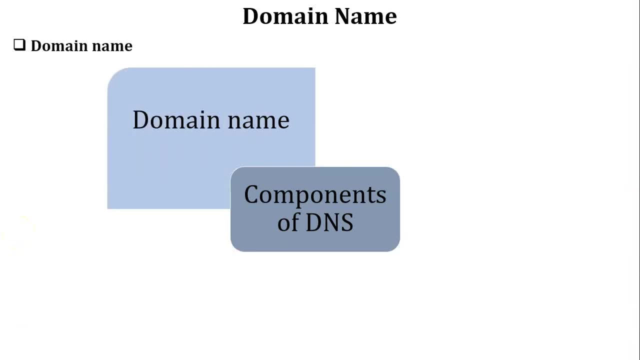 In detail, one by one. First component of DNS is domain name. Domain or domain name means location of website. We all know that web pages of our website is stored on particular server And server is connected with particular domain. So domain or domain name means location of website. 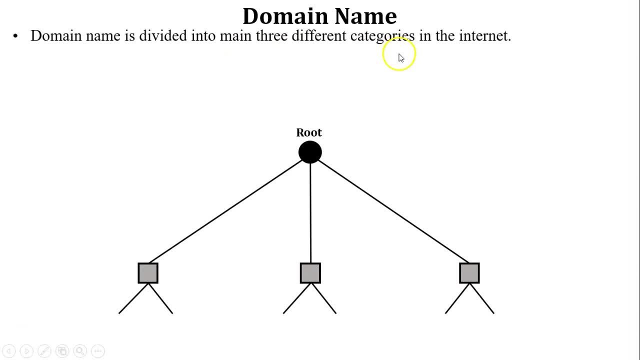 Next, domain name is divided into main three different categories in the Internet. Now see in this diagram: the first domain name is generic domain, The second one is control domain And the third one is inverse domain. So these three are the main domain of the DNS in the Internet. 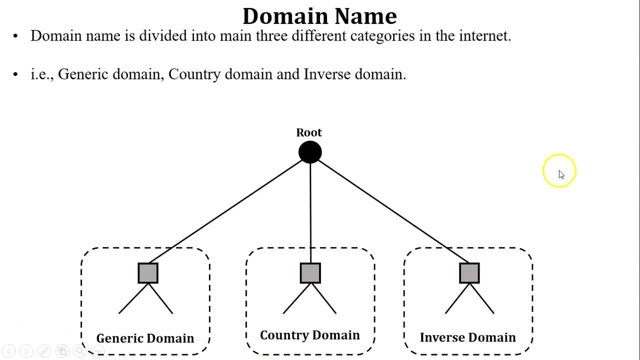 All the domain and subdomain in the Internet is connected with any one of this domain. Next, each node in the tree defines a domain. Now see in this diagram. this is the tree structure: Root is the parent node, Generic domain, country domain and inverse domain is the child node of the tree. 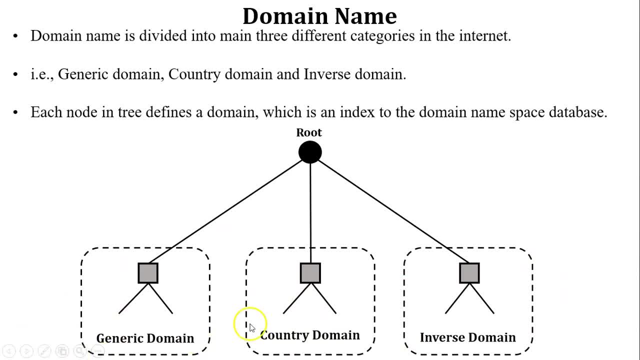 So these three are the first child node, So it is called the top level domain. in the DNS Each domain is an index to the domain namespace database. We have already discussed all the domain and subdomain in the Internet is connected with any one of this three domain. 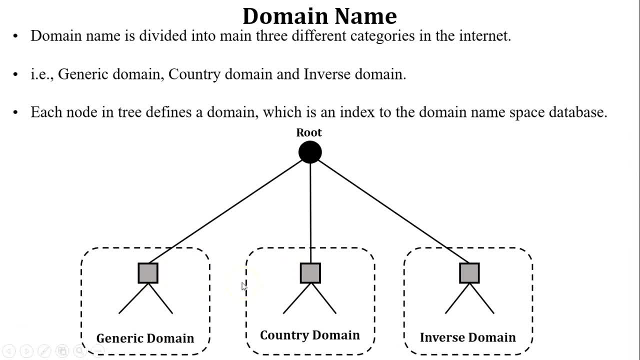 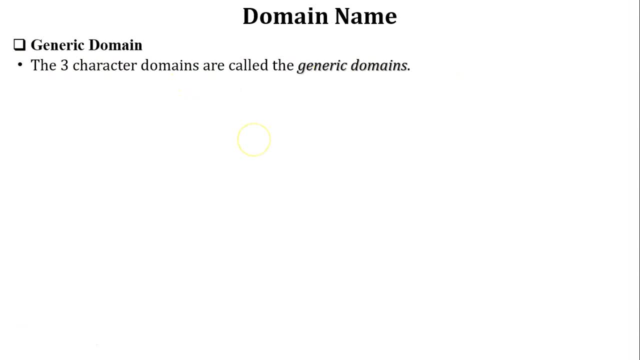 Let's discuss this three domain one by one in the detail, with example. The first domain is generic domain. The three character domains are called the generic domains, But nowadays two character and four character domains are also available in the generic domain. Next, generic domain labels are as follow: 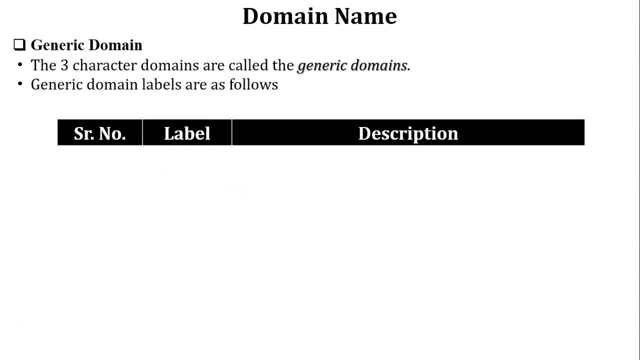 Now see this table to understand the generic domain levels. First one is com, for the commercial organization. The second one is edu, for the educational organization. The third one is gov, for the government organization. The fourth one is int. it means the international organization. 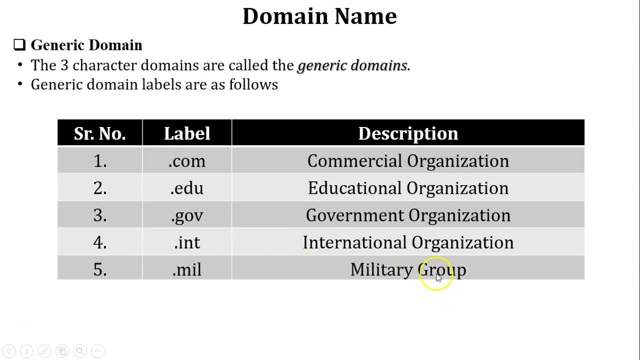 The fifth one is mil: it is used for the military group, The next one is net: it is used for the network support centers, And the next one is org- It is used for the nonprofit organizations. So here there are the some of example of the generic domains. 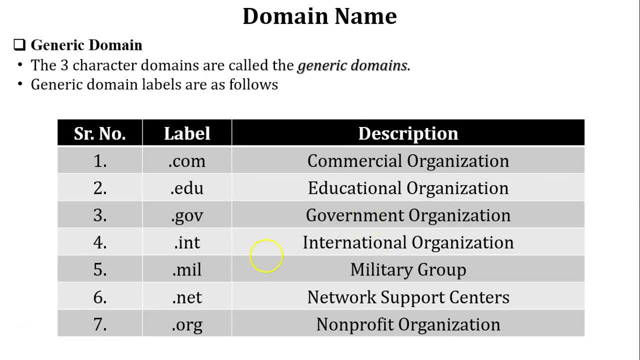 Also many more generic domains are available in the DNS and we all know that our website is ended with this particular labels. If this kind of label is present in our website, it means our website is belongs to the generic domain. Let's take one example to understand the generic domain in the detail. 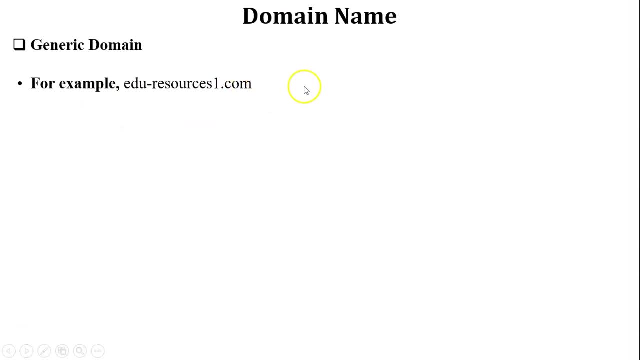 For example, I am accessing one website, eduresources1.com, So how can I access this website? now understand with tree structure of the DNS. In the DNS tree structure, we all know that the first node is root node. Root node is connected with three different domains: generic domain, country domain and inverse domain. 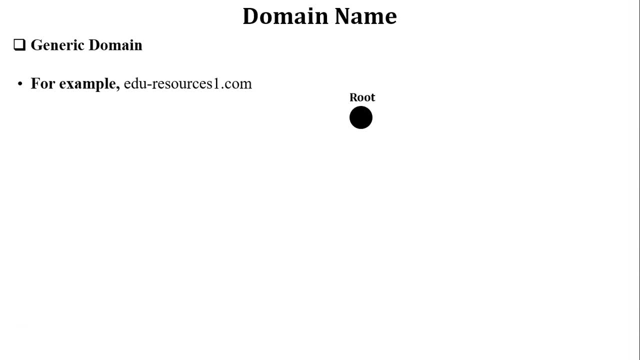 So here we discuss about the generic domain only. So root node is connected with the different generic domains, like educomgovmilnet. So this, all the domain, are connected with the root node. It is called as the top level domain. So here in our example our website is connected with com domain. 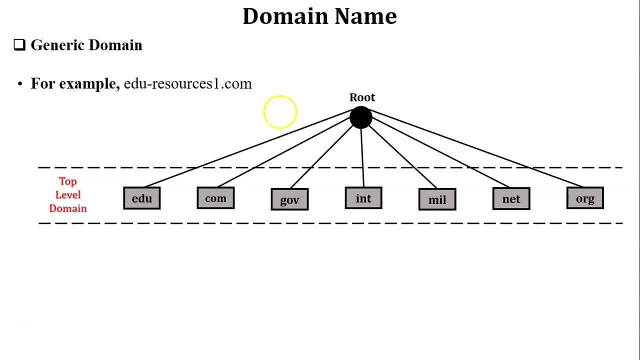 It means our website is belongs to the generic domain, So our website top level domain is com. All the top level domains are connected with respected subdomains. That is called second level domain. So in this example, our URL is eduresources1.com. 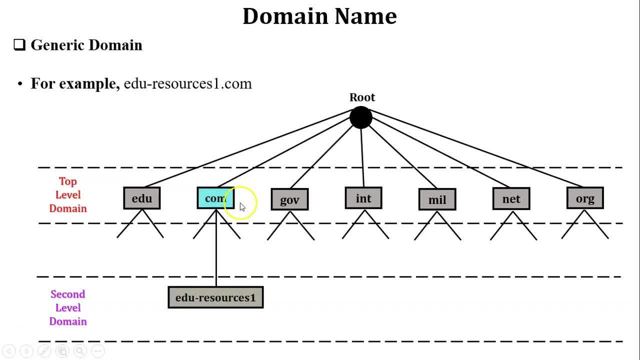 Here com is the top level domain and eduresources1 is the second level domain. So it means The URL is written in the inverse DNS tree structure. Now see in this diagram eduresources1.com. So this is the example of generic domain. 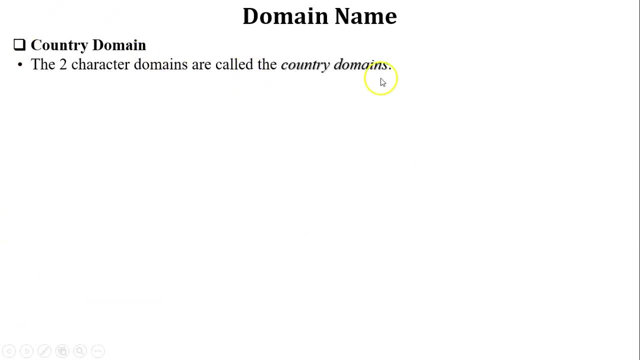 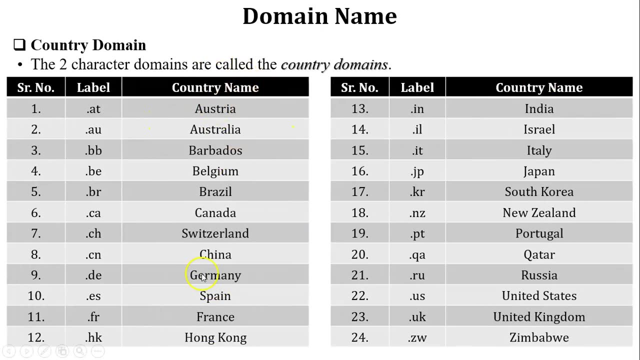 Next domain is country domain. The two character domains are called the country domains. Here I have show the some of the example of the country domains. Now in this third column, this is the country name and this is the label of the country domains. Like Austria, it means at Australia, it means au. like India is in. 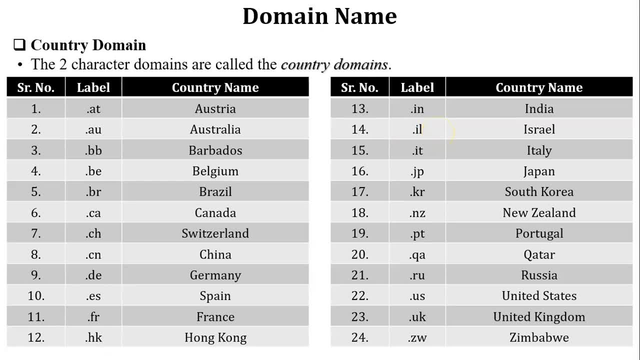 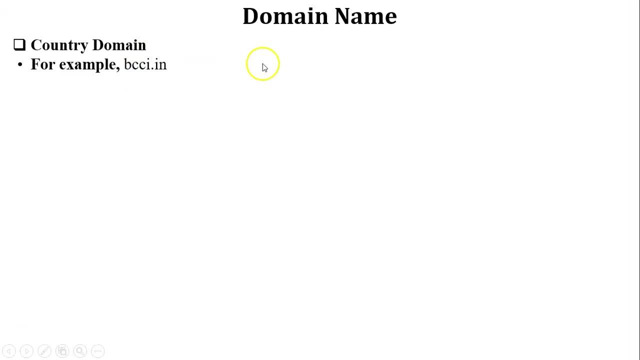 Israel, il. So here these are the some example of the country domains. In country domain all the country names label are two characters. Let's take one example to understand the country domain in the detail. For example, there is one web URL, bcciin. 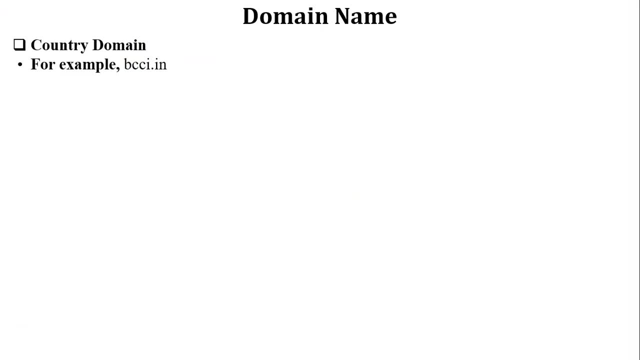 So let's understand how it belongs to the country domain. So first of all, there is a root node in the DNS tree. Root node is connected with the main three domains: Generic domain, country domain and inverse domain. Here we are discussing about the country domain. 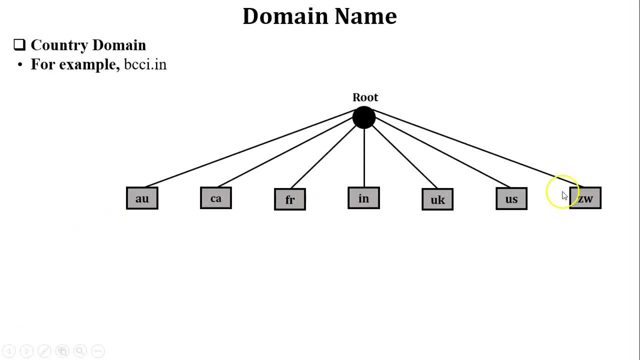 So here root node is connected with some of the country domains. So this all are country domain is the top level domain. in the DNS This all top level domains are connected with the respected sub domain. It is called the second level domain. So here in our example top level domain is in: 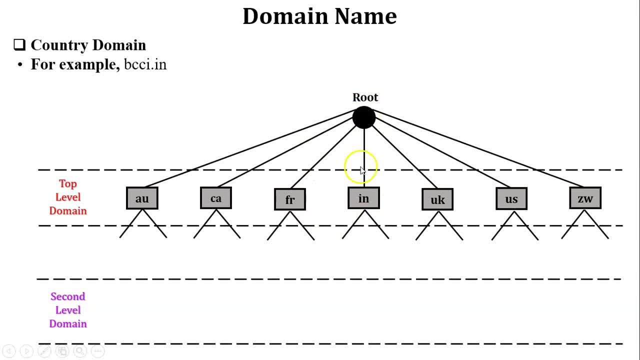 So now see in this diagram: in is the connected with the root node Because in is the top level domain. Now second level domain is bcci, So it means our website is bcciin. So now see in this diagram: bcciin is the connected with the root node. 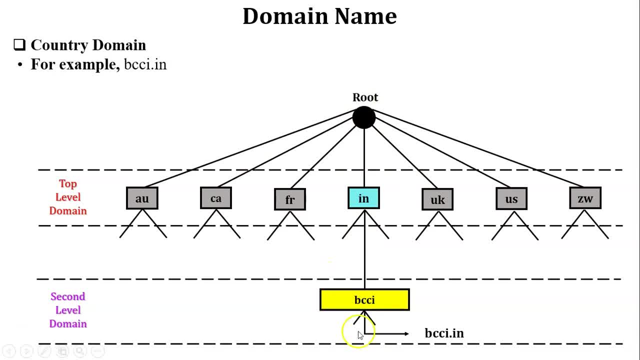 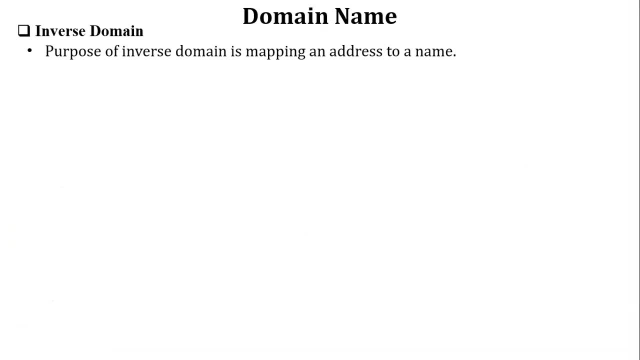 So now you can see over here in this diagram, web URL is written in the inverse tree domain structure. Next domain name is inverse domain. The purpose of inverse domain is mapping an IP address to a website name. So let us take one example to understand the inverse domain. 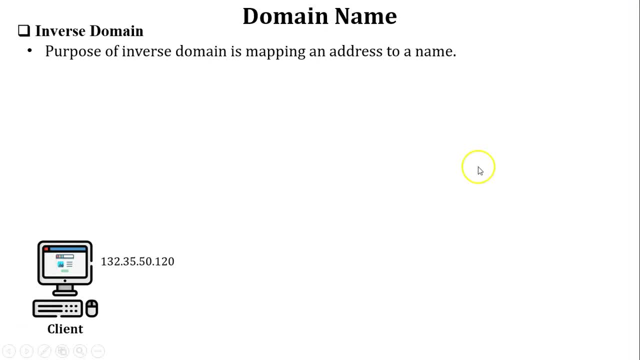 There is one user. User want to access a website through the IP address. So first of all user will send this IP address to the root server. So root server check the IP address in the list of IP addresses But root server cannot map this IP address to the website name. 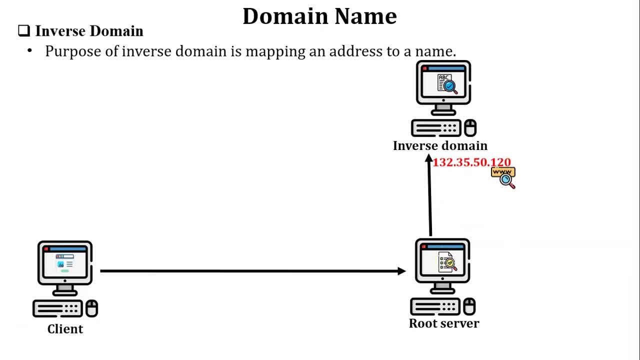 So root server send this query to the inverse domain. So this query is called a pointer query or an inverse query. So how inverse domain evaluate this query? So we all know that in DNS root node is connected with three main domain. The first one is generic domain. 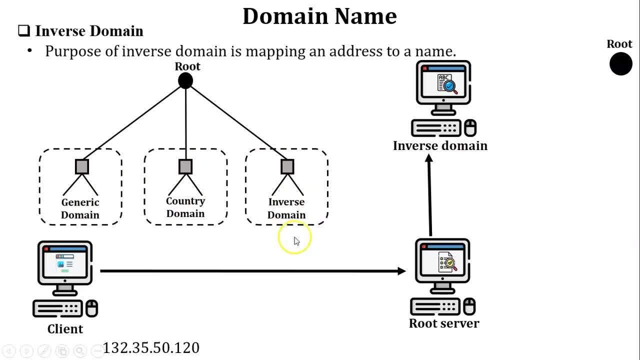 The second one is country domain And the last one is inverse domain. So here we are discussing the inverse domain In inverse domain. the top level domain is ARPA, So root node is directly connected with the ARPA domain. The ARPA is connected with the second level domain in the inverse domain is in address. 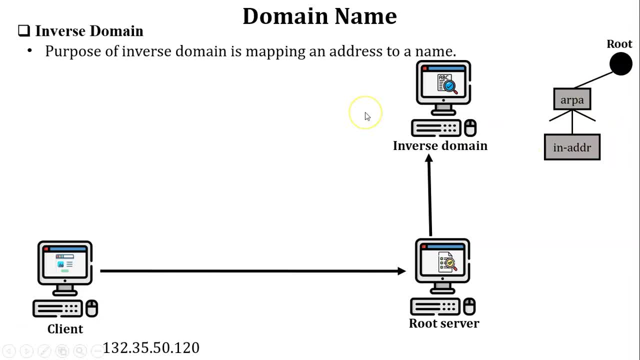 Meaning the in address is inverse the address, So rest of the node. define the IP address: 132.35.50.120- So IP address is written in the inverse DNS tree structure. 135.132-inaddress-arpa, So inverse domain. evaluate that IP address and map with the website name. 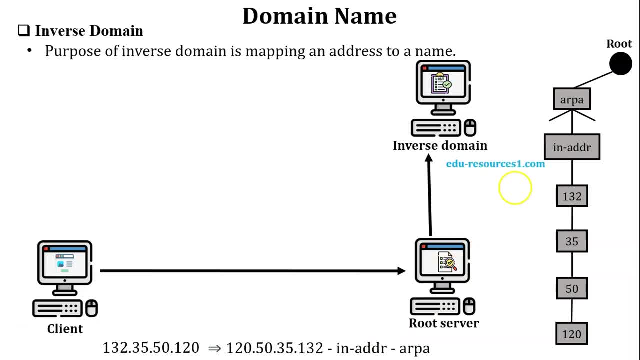 For example, this IP address is mapped with the web URL eduresources1.com. So now inverse domain. pass that URL to the root server, Because in this web URL the top level domain is com. It means the website belongs to the generic domain. So now see this diagram Here: generic domain and. 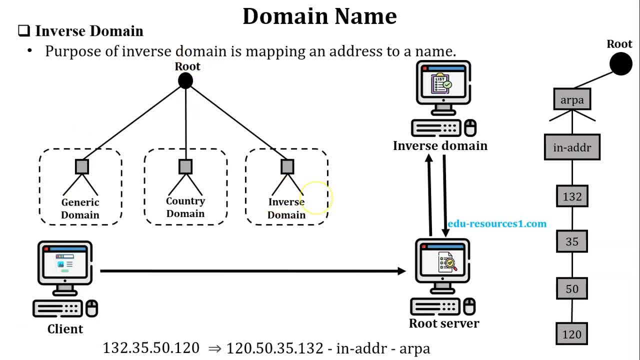 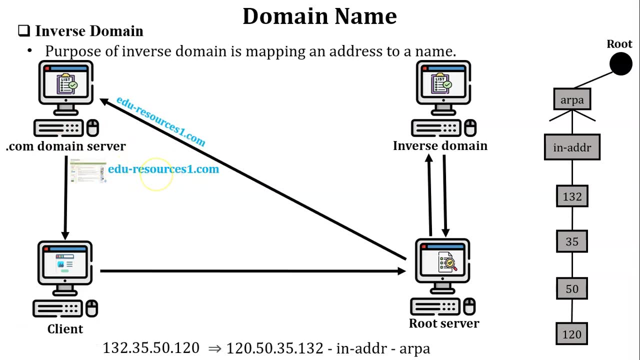 inverse domain. both are connected through the root node, So inverse domain cannot send URL directly to the generic domain. Now, root server. pass this URL to the com top level domain. Top level domain: check the second level domain, eduresources1.. It means the web server of that website. So after: 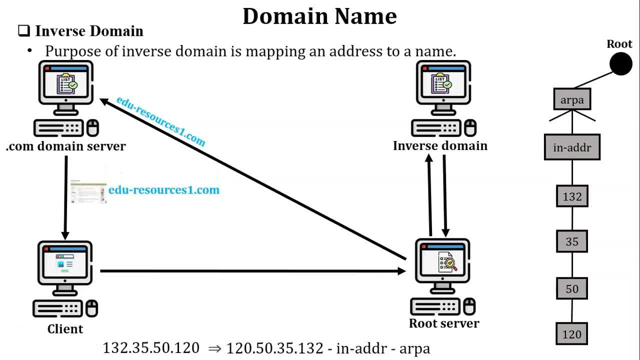 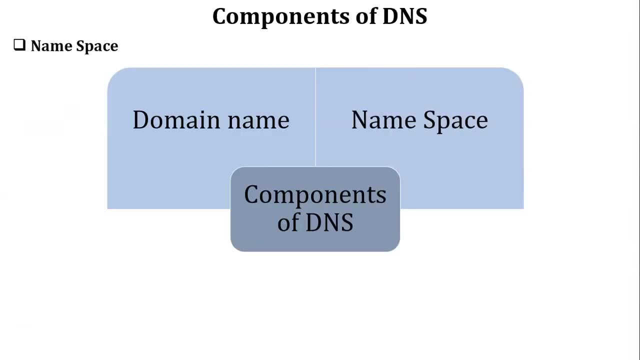 that web server send requested page to the user and the website will display on the user's web browser. So this is the actually working of inverse domain. What I have explained here in inverse domain is written over here. You can read from this slide also. Next component is namespace. There are two. 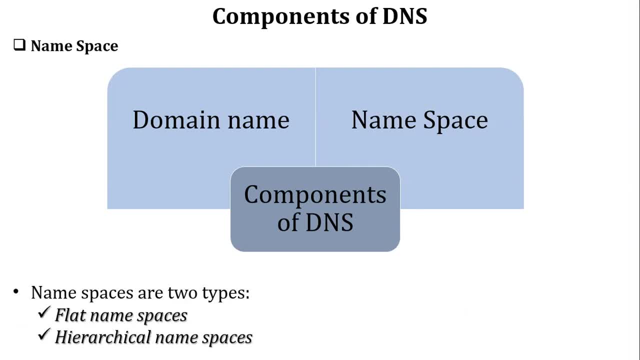 types of namespace. The first one is flat namespace and the second one is hierarchical namespaces. In flat namespace, all the nodes are directly connected to the root node, So there is no structure. in the flat namespace, In hierarchical namespaces, all the nodes are connected with different partitions. 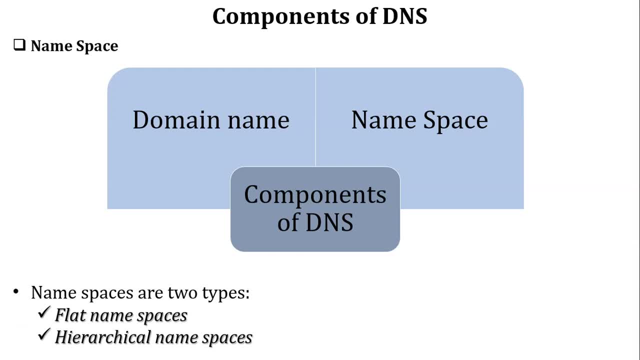 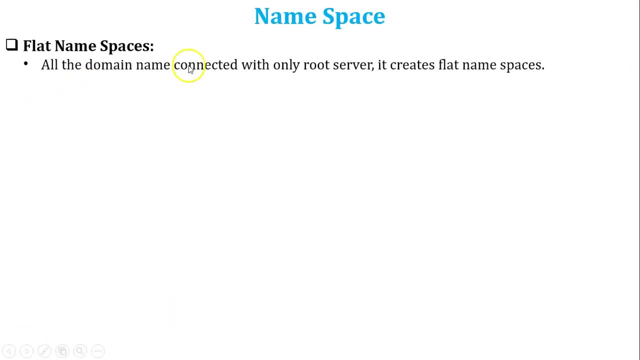 like top level domain, second level domain, third level domain. So now discuss both the namespaces one by one. The first one is like the first one is flatNamespaces In flat namespaces, all the domain name connected with only root server. It creates a flat namespaces and all the remaining 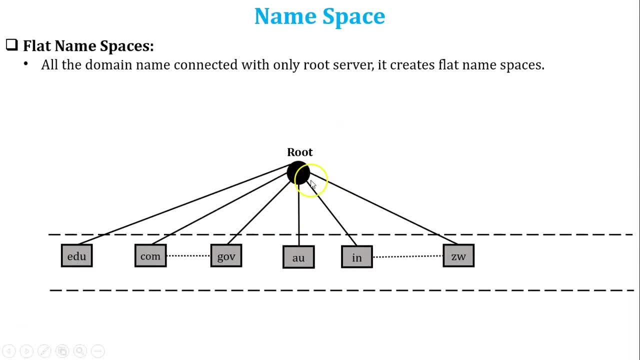 nodes are directly connected to the root node. that is called the flat namespaces. Next, there is nice structure in the flat namespaces because all the nodes are connected to the root node. For example, new node is added in the internet, It is directly connected to the root node. 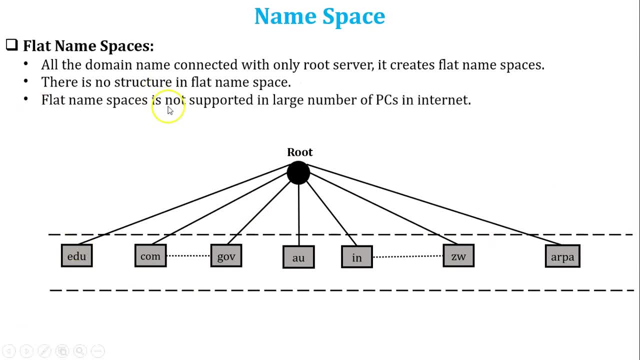 Next, flat namespaces is not supported in a large number of places in the internet, As I said earlier in the internet. nowadays in internet there are millions of PCs are connected with each other through the DNS, so whenever large number of PCs in the internet, at that time flat namespaces are not working. next in flat namespace. 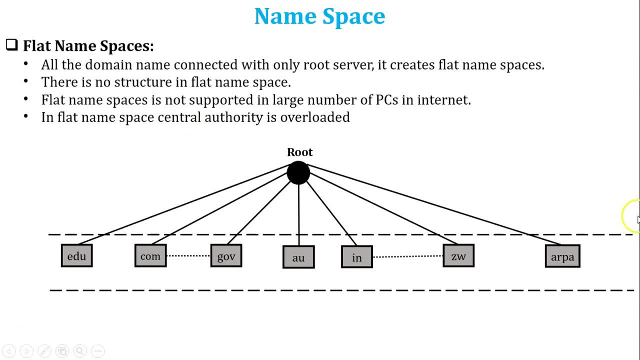 central authority is overloaded. so we have already discussed about that. all the nodes in the internet is connected with the root node. so whenever new node is added into the internet it is directly connected with the root node. so central authority is overloaded in flat namespace. there is no further division. 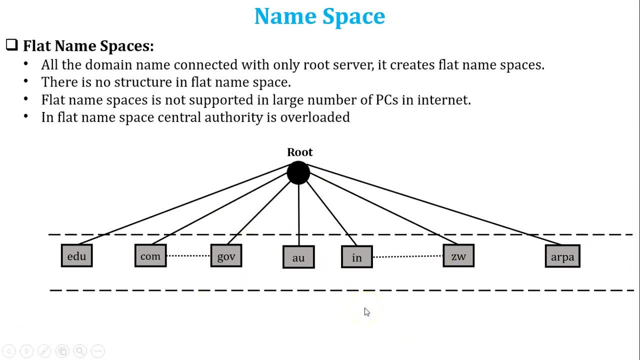 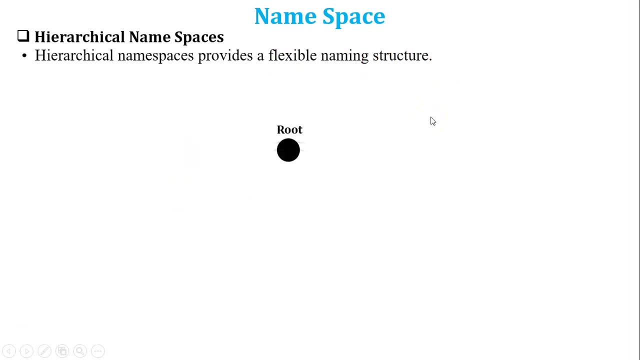 of the different domains, like generic domain, country domain and inverse domain, because all the nodes are present in the top-level domain. to overcome the limitation of the flat namespace, hierarchical namespaces is used. so in hierarchical namespace provide a flexible naming structure. now see in this diagram: root node is connected with the different nodes in the internet. the 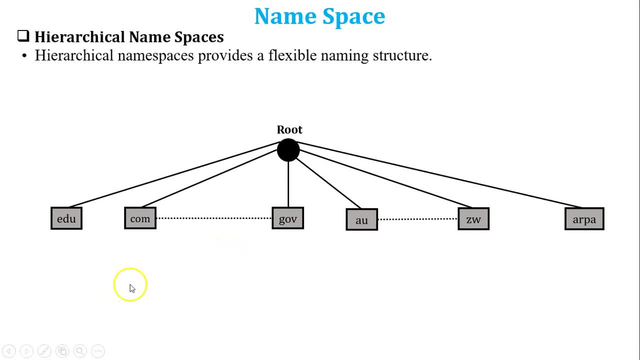 nodes that are directly connected to the root node in the internet are connected to the root node, and the nodes that are directly connected to the root node is in the hierarchical namespaces. it is called the top-level domain. next the namespaces is partition at the top-level domain. next the top-level domains are: 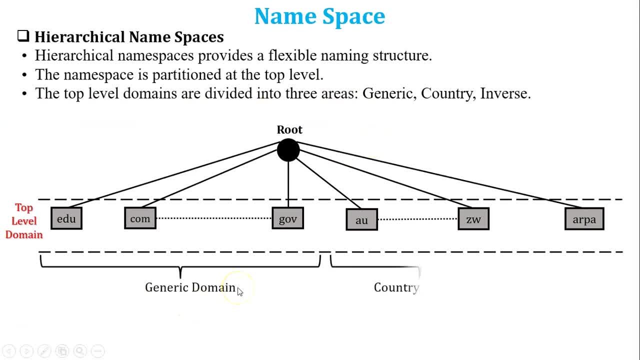 divided into the three areas. the first one is generic domain, the second one is country domain and the third one is inverse domain. now, top-level domain is further divided into the second level domain. so this diagram shows the hierarchical namespace in the DNS. for example, our website is edu resources one. 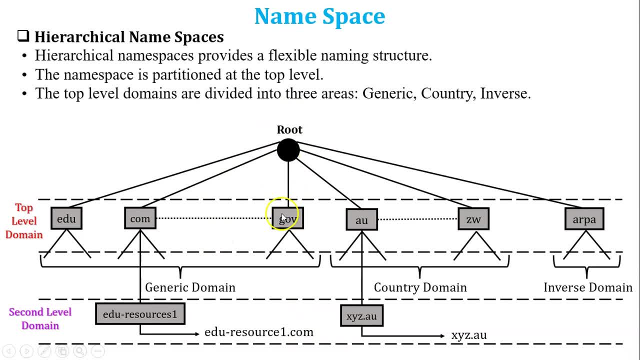 dot com in hierarchical namespace, root node can easily find the website because root node check the top-level domain in the website URL. so in our example the website URL top-level domain is dot com. it means our website is belongs to the generic domain and the second level. 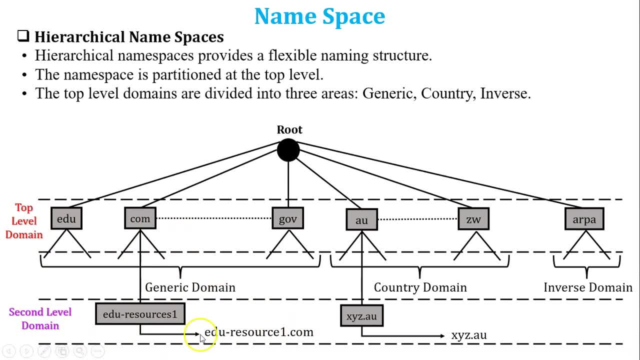 domain is edu resources one. so web URL is written in the inverse DNS tree structure: edu resources one, dot com, the same as. another example is the country domain XYZ, dot au. so in this URL, a root node, check the top-level domain. so here top-level domain is dot au, so it means dot au s belongs to the country. 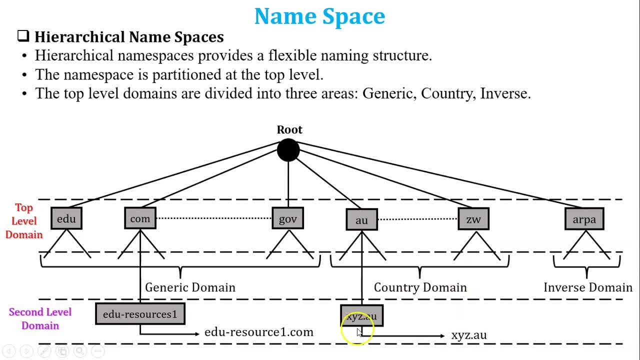 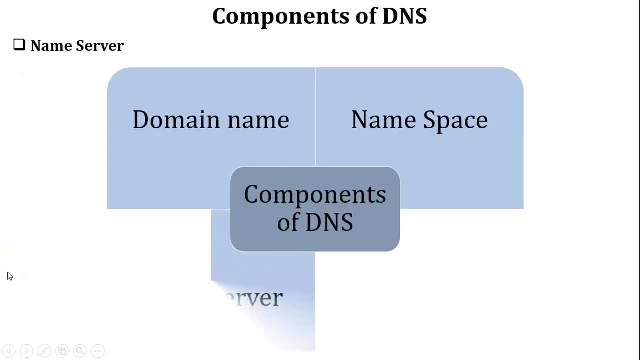 domain and the second level domain is XYZ, so or web URL is XYZ, so using the hierarchical namespaces in the Internet, DNS can easily map the web URL with the IP address with the immediate response to the user. next component of DNS is DNS name server. so, first of all, what is name server? a DNS name server is a server that store the 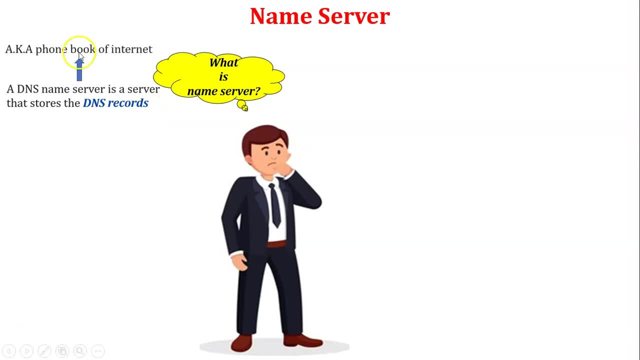 DNS records. So name server is also known as the phonebook of internet. Next, which kind of records has been stored in name server? Name server store address record, name server record and the mail exchanger record and also store the many more records. Next, what is the purpose of name server? 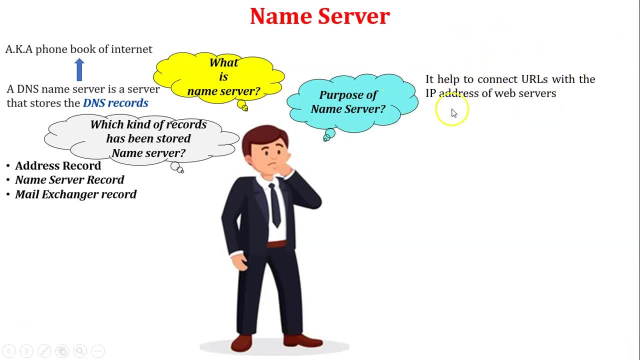 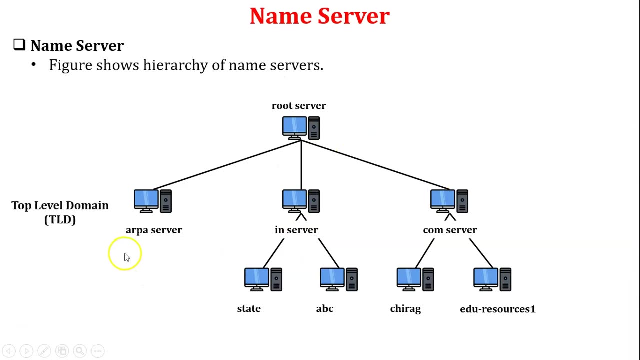 So name server help to connect URLs with the IP address of the web servers. Next server has some authority and also responsible for the operation which is performed in the DNS. Next figure shows the hierarchy of the name server. So in this figure, root server is connected with the top level domain. 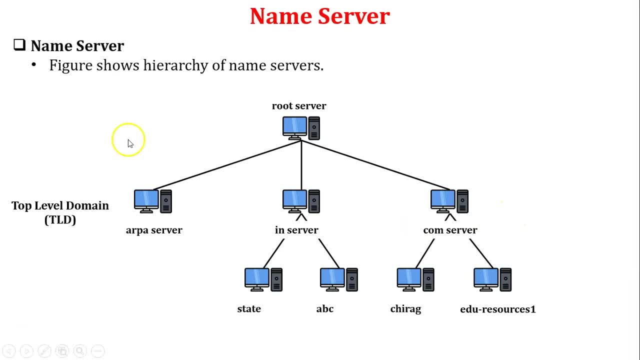 arpa server in server and com server. So here in and com top level domain is connected with the some secondary level domain. For example, I want to access a one website, eduresources1.com. So in this website URL, eduresources1 is the second level domain, which is: 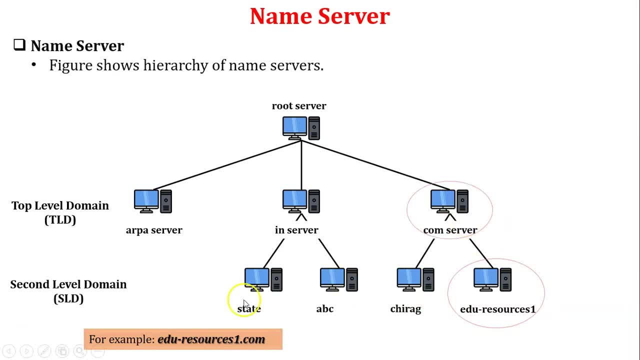 connected with the top level domain. So in this website URL, eduresources1 is the second level domain which is connected with the top level domain. So our web URL is connected in a inverse DNS tree structure. Now see in this diagram, eduresources1 and which is connected with the com. 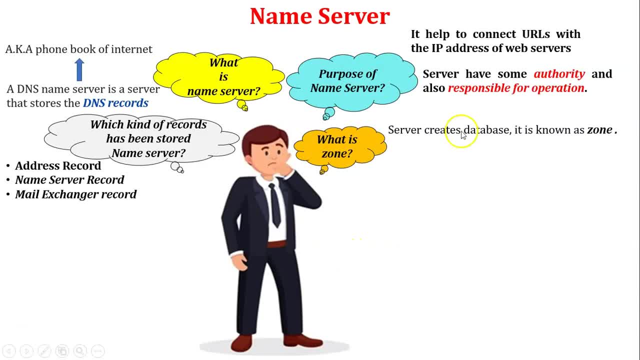 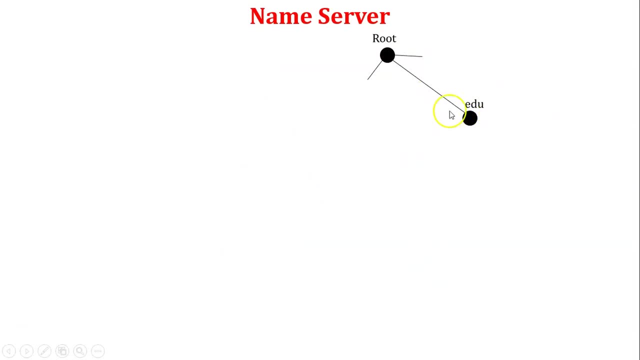 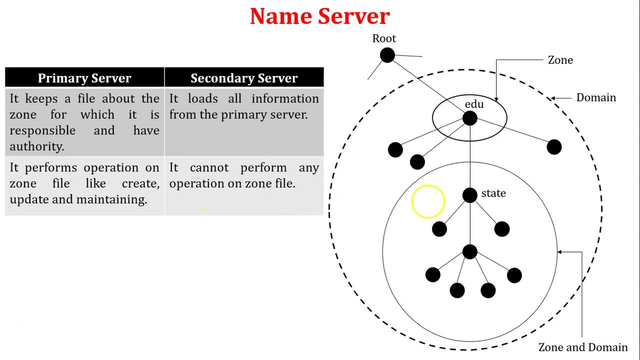 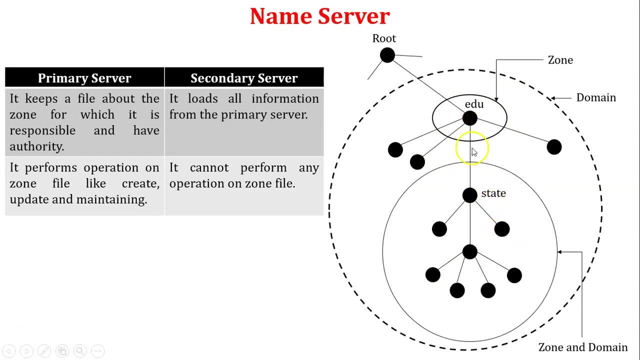 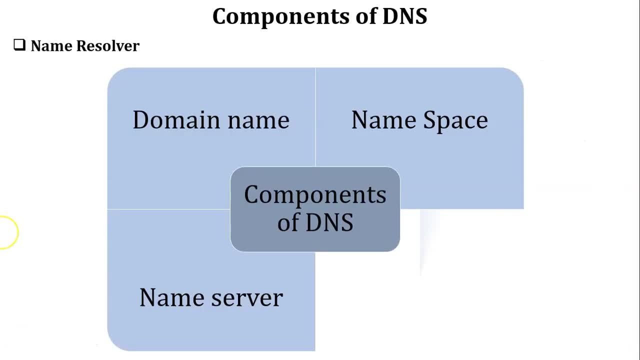 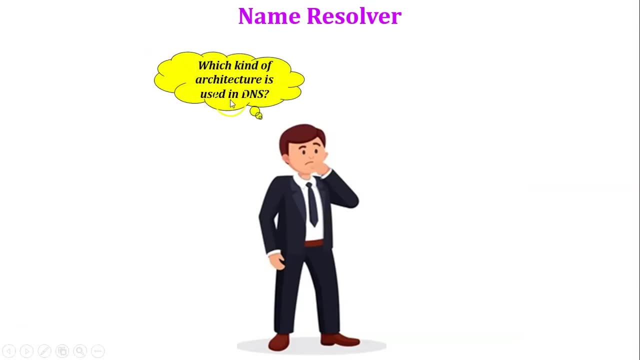 the information. at that time it loads all the information from the primary server. so this is the primary server and secondary server inside the dns name server. next component is name resolver. so before discuss about the name resolver, there is one question: which kind of architecture is used in dns? there is client server architecture is used in the dns. next, what is name resolver? name? 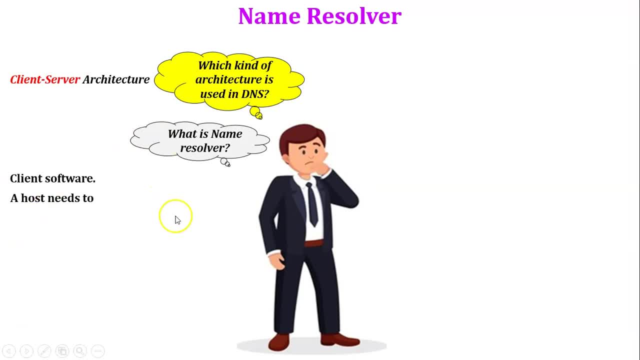 resolver is one kind of client software. when host needs to mapping domain name to ip address and ip address to the domain name, at that time name resolver is used. next, how many types of name resolver? there are two types of name resolver. the first one is mapping a domain name to an address. 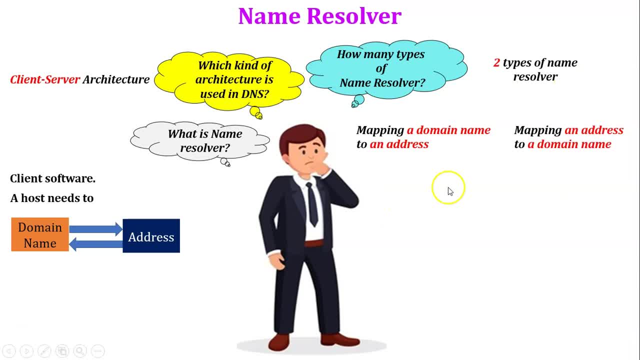 and the second one is mapping an address to a domain name. so there are two different method are used for the name resolver. the first one is the recursive method and the second one is iterative method. so now, first we discuss the types of name resolver and then discuss recursive and iterative method. 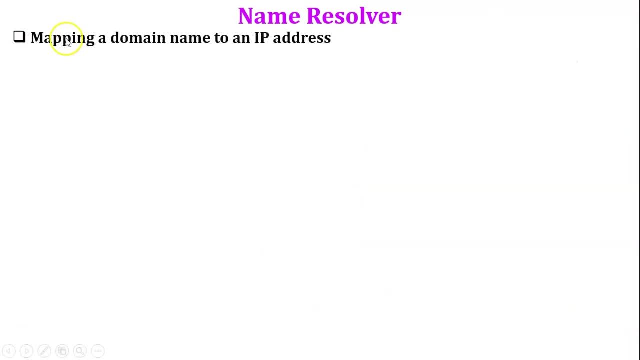 so let us understand the types of name resolver. the first type is mapping a domain name to an ip address. so let us take one example to understand the first type: mapping a domain name to an ip address. for example, there is one user. user want to access one website. the website url is wwwedu. 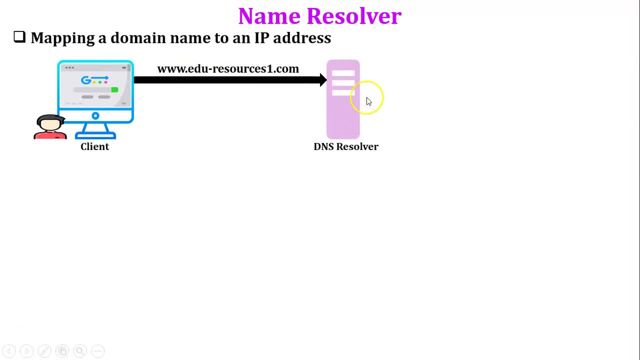 resources: one dot com. so client browser. pass this url to the dns resolver. dns resolver: pass this url to the dns server. dns server: map this url with the ip address of that web server and pass that ip address to the dns resolver. then dns resolver pass this ip address. 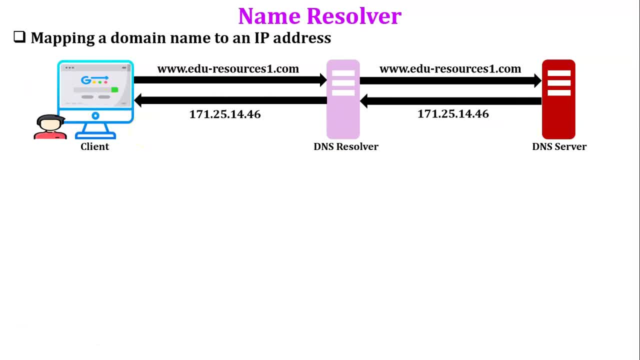 to the user's browser. so now user's browser access that website through that ip address. we all know that there are three types of domain are connected to the dns root node: the first one is generic domain, the second one is country domain and the third one is inverse domain. so in this, 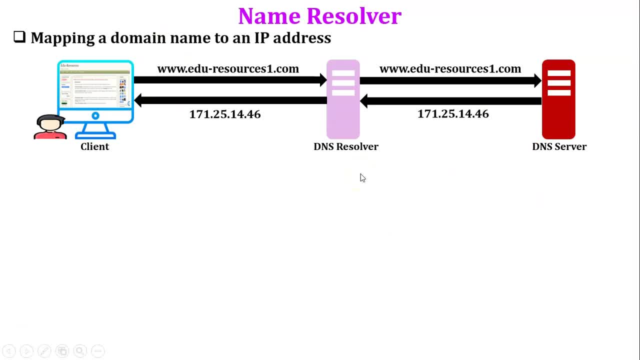 mapping technique. dns server map domain name to an ip address, either generic domain or country domain, next types of the name. resolver is mapping an ip address to a domain name. so let us take one example to understand this mapping technique. for example, there is one user user want to access a. 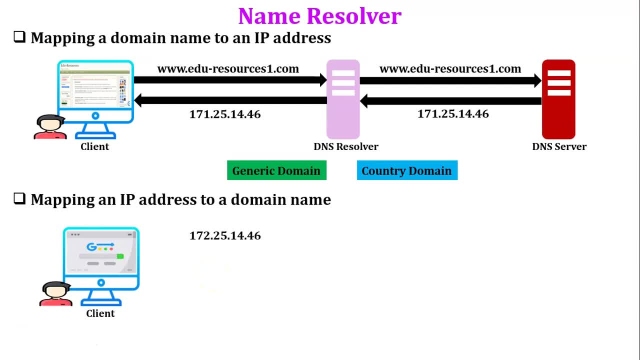 website through the ip address. so first of all users browser send that ip address to the dns resolver. dns resolver send this ip address to the dns server. so dns map that ip address to the dns resolver. so dns map that ip address with particular web server and pass this web server. 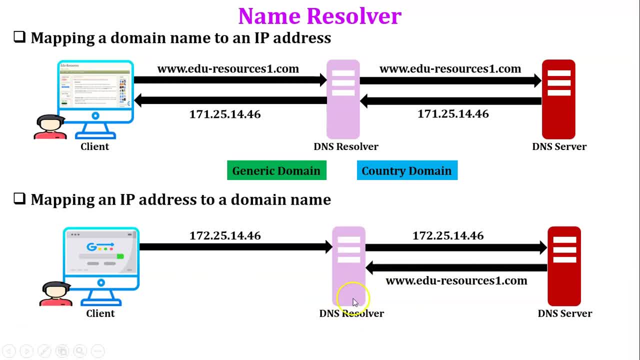 name to the dns resolver and dns resolver pass this web server name to the user's browser. so now user's browser is connect to that particular web server and the website is open at the user's browser. so in this mapping technique, dns server use inverse domain, so using the inverse domain. 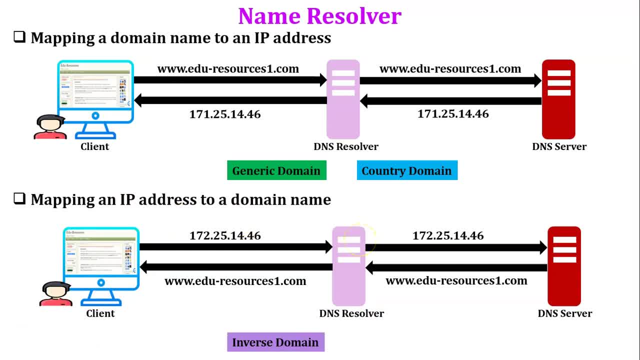 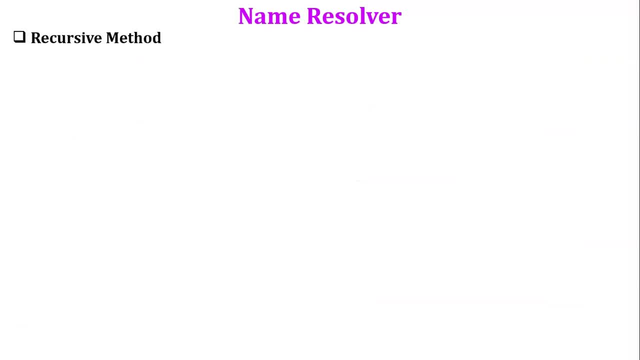 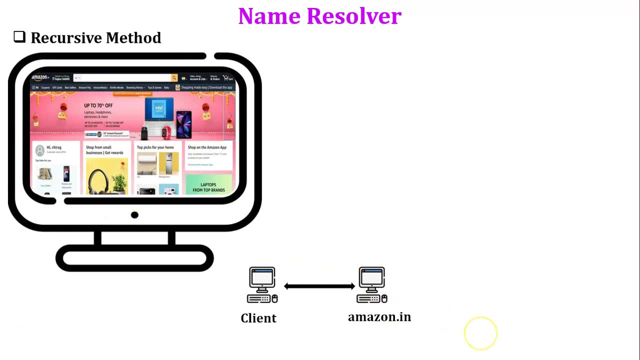 ip address is mapped with the domain name. now let's discuss recursive and iterative method one by one. first of all, i will discuss recursive method. let's take one example to understand the recursive method. there is one user. user is accessing a website- amazonin- so after some time, user want 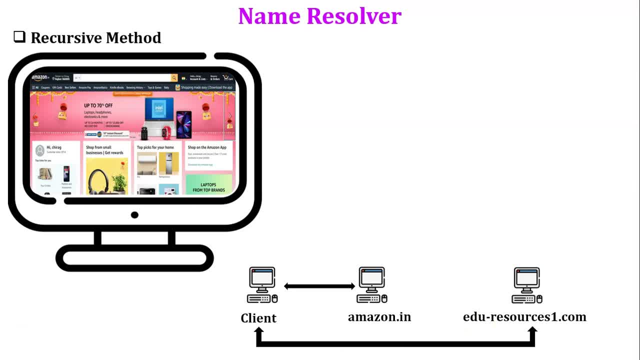 to access another website, eduresources1.com, but user cannot directly access that website, so user send a request to the web server which is currently accessing by the user. so here, user currently accessing the amazonin web server, so amazonin web server is trying to evaluate. 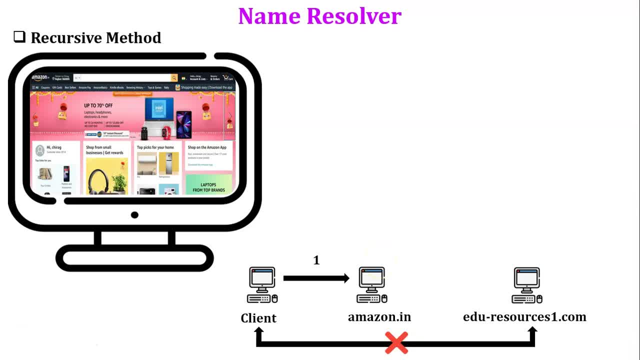 that query. but this query is not resolved by the amazonin web server, so this web server pass this query to the upper level authority here. upper level authority is the top level domain dot in. so top level domain, try to evaluate that query, but it cannot be evaluated by the 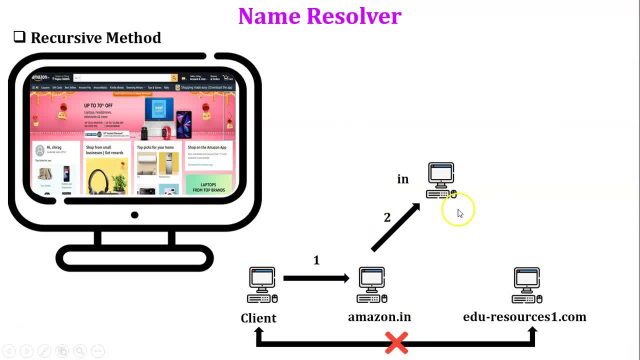 top level domain. so top level domain dot in. pass this query to the upper level authority root node. so first of all, root node. check the top level domain in the url. so here: top level domain dot com. so root node. pass this query to the dot com top level domain. so top level domain check. 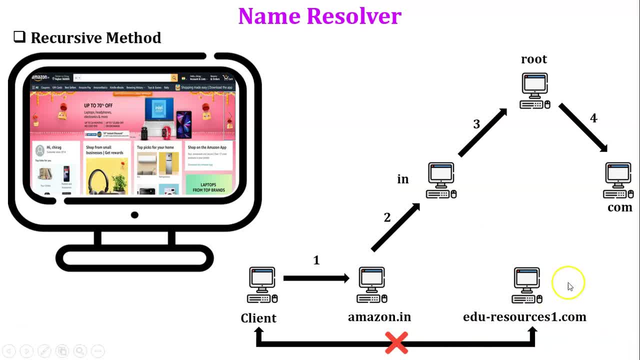 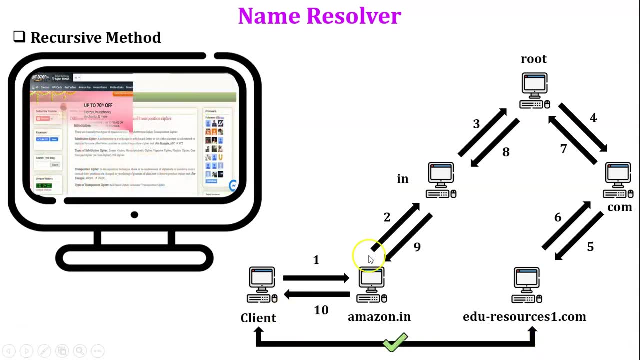 the second level domain in that web url. the second level domain is edu resources one, so top level domain. pass this query to the second level domain, edu resources one. when the query is finally resolved, the response travel back until it finally reaches the requesting client and now client can access. 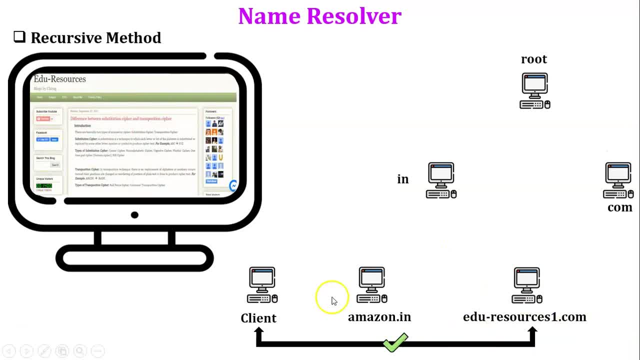 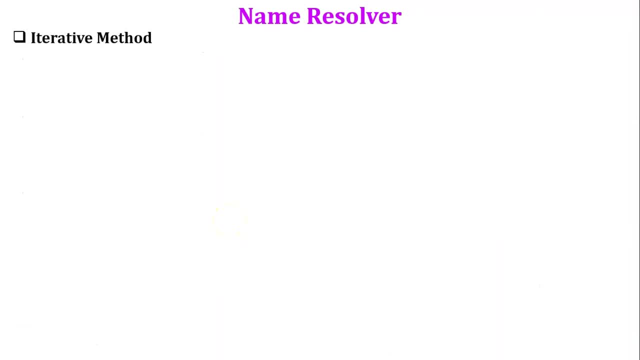 that website, edu resources one dot com. so this is called the recursive method. now what i have in the recursive method you can read from this slide. the next method is iterative method. let us take one example to understand the iterative method. there is one user. user is currently. 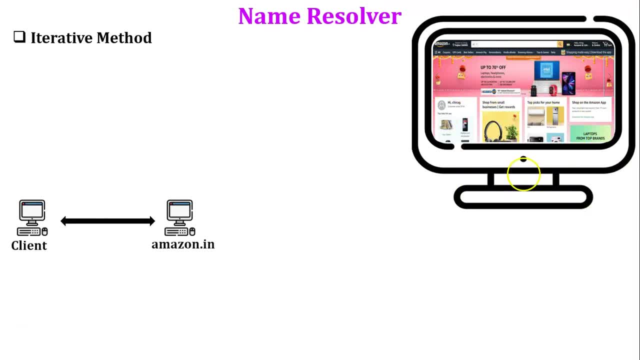 accessing the website amazonin. it means user is connected with the web server amazonin. so after some time user want to access another website, edu resources 1.com, but user cannot access that website directly. if the client does not ask for a recursive answer, the mapping can be done. 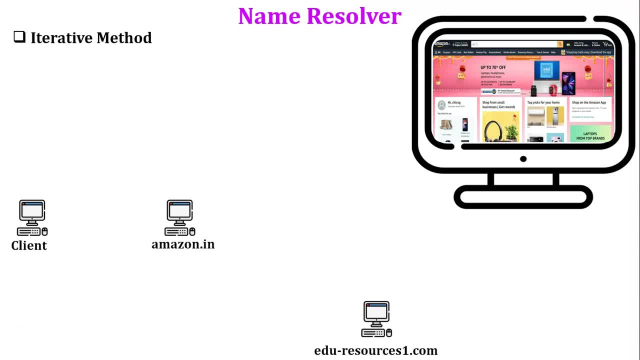 it will not be able to access that website directly. if the client does not ask for a recursive answer, the mapping can be done it iteratively. so client send a request to the currently accessing web server. so here currently accessing web server is the amazonin, so here amazonin web server cannot evaluate the query. 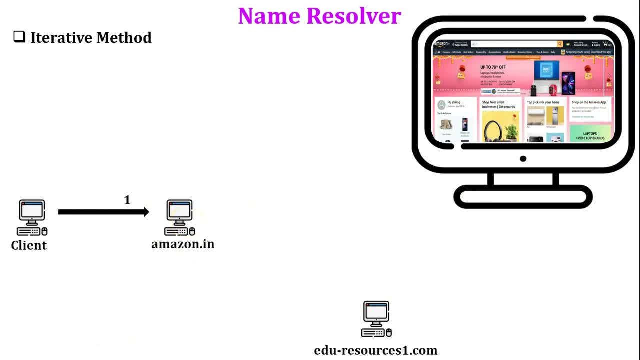 so amazonin web server provide the ip address of the upper level authority to the client or user. so user pass this query to the upper level authority. here upper level authority is the top level domainin. so again, top level domainin cannot evaluate that query and provide the upper 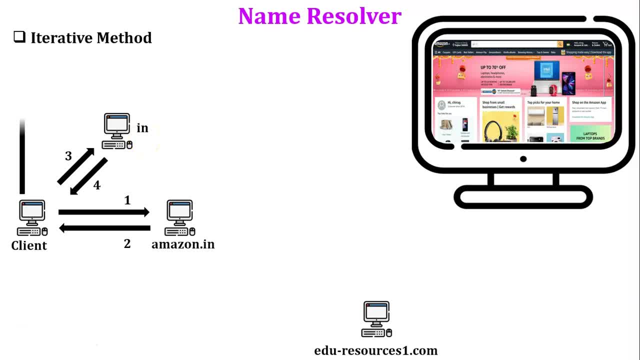 level authority ip address to the client. so now client send a query to the root node. so root node check the url and find the top level domain here. top level domain is com, so root server provide the ip address of the top level domaincom. so root server provide the ip address of the top 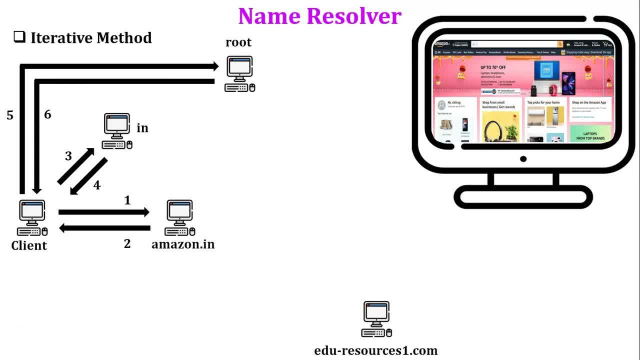 level domaincom to the user. so now user has the ip address of the top level com domain. so user pass this query to the top level domaincom. so here top level domaincom check the second level domain. so here second level domain is edu resources one. so top level domain. 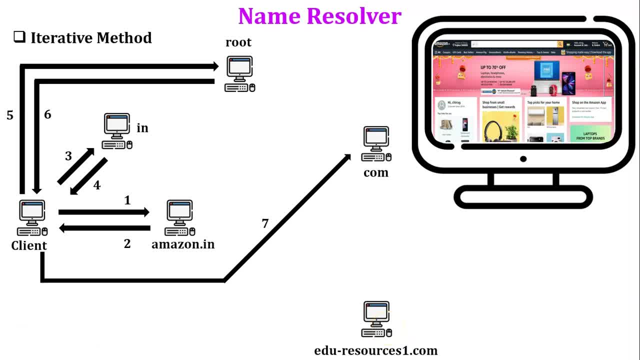 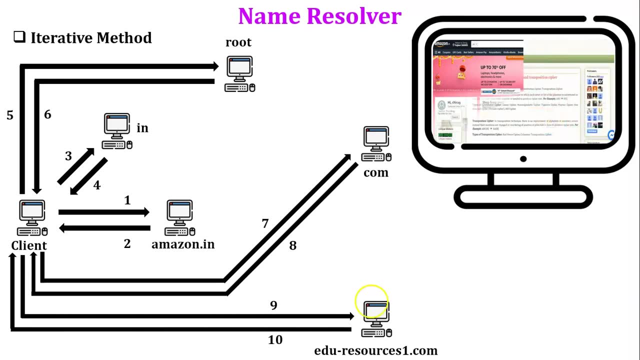 provide the ip address of that web server, or we can say second level domain, to the user. so now user send a request to that ip address, edu resources, onecom. so now user send a request to that web server ip address so that web server provide the requested file to the user and user. 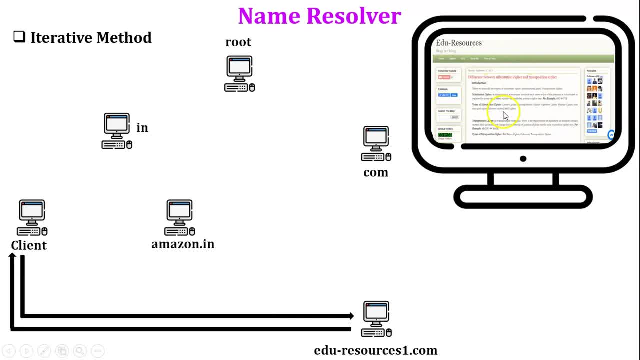 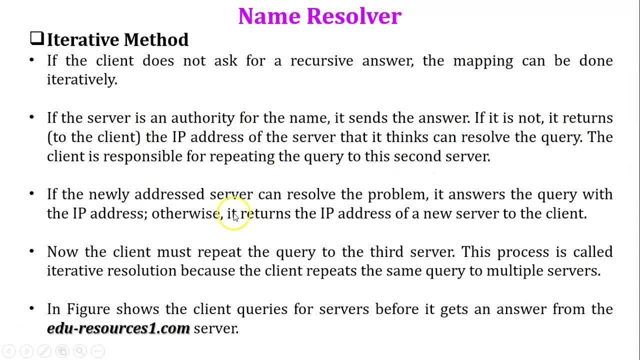 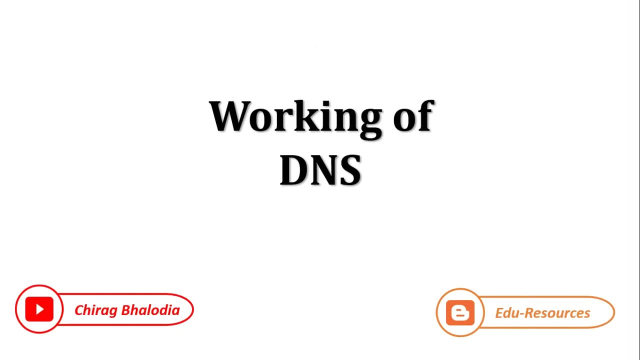 user can access the website eduresources1.com. so this is called the iterative method. so what i have discussed over here is written in this slide. you can read from this slide. next, working of dns. let us take one example to understand the working of dns. there is one user. user want to. 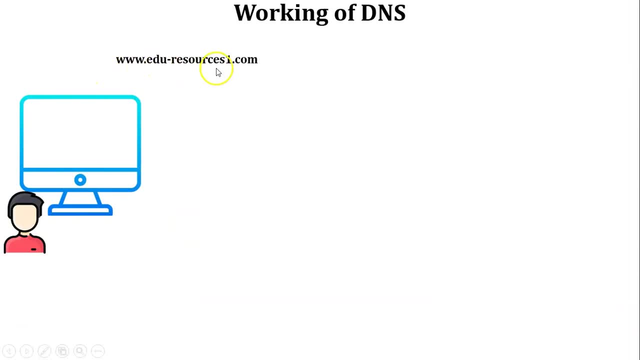 access a website- wwweduresources1.com. so first of all, user enters the url into the web browser. web browser sends this url to the dns resolver. the purpose of dns resolver is mapping website name to ip address and ip address to website name. now dns resolver send this url to the root server. 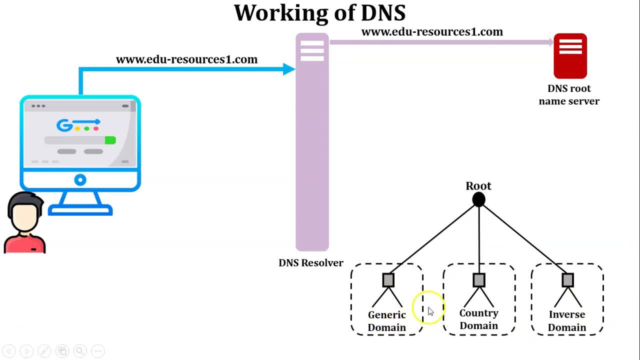 root server is connected with three main domains: generic domain, country domain and inverse domain. so here we all know that the purpose of inverse domain is mapping ip address to the domain name. but in this example dns resolver sent the website name to the dns root server. so here root server will not contact to the